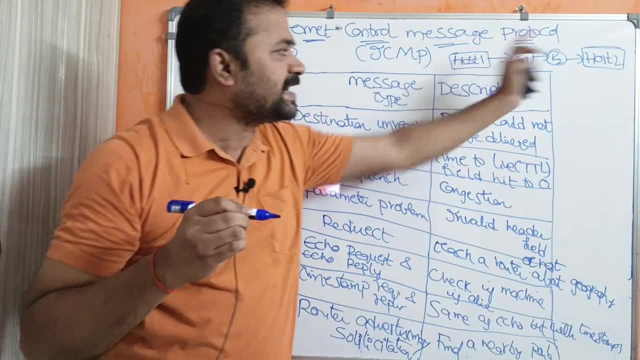 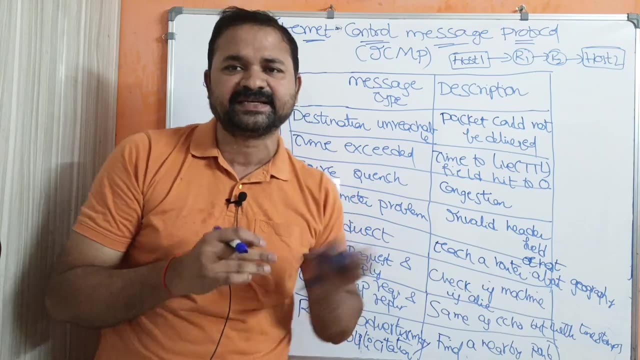 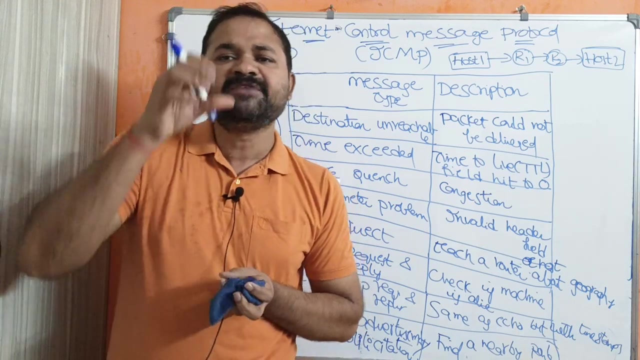 here host 1 is transmitting a datagram to the host 2.. But during the transmission there may be a possibility that the datagram or packet may be lost. But here the problem is: if the packet is lost, then the packet may be lost. So if the packet is lost, then the packet may be lost. So if the 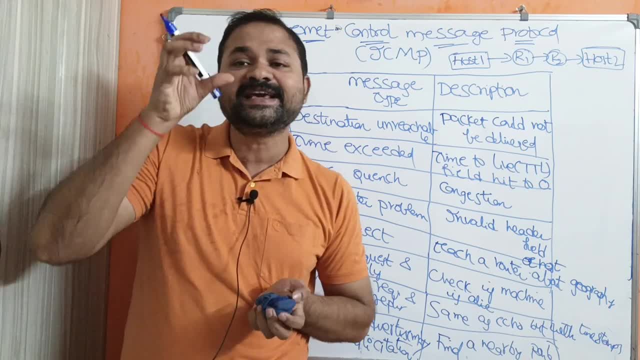 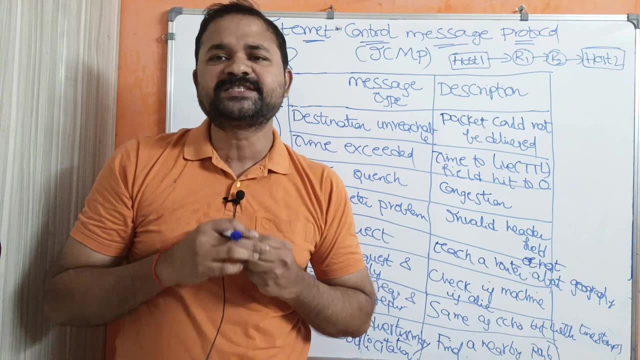 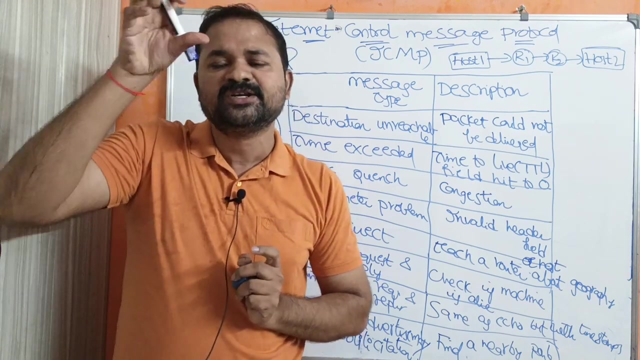 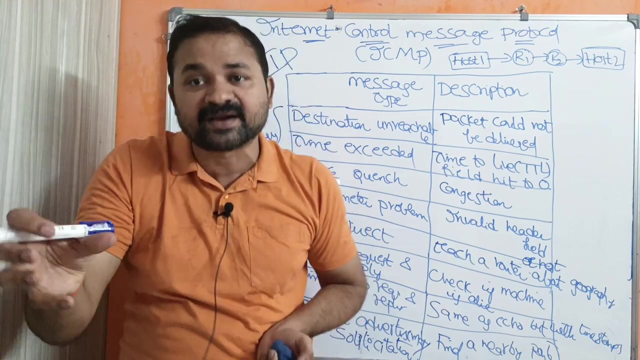 packet is lost due to any problem, then there is no way to report to the source host in IP. So we can say that IP is an unreliable protocol. Why? because if the packet is lost due to any problem, then there is no way to report about that error to the source host. So in order to solve this, 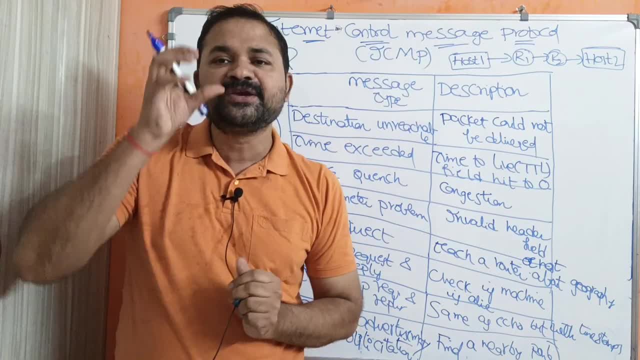 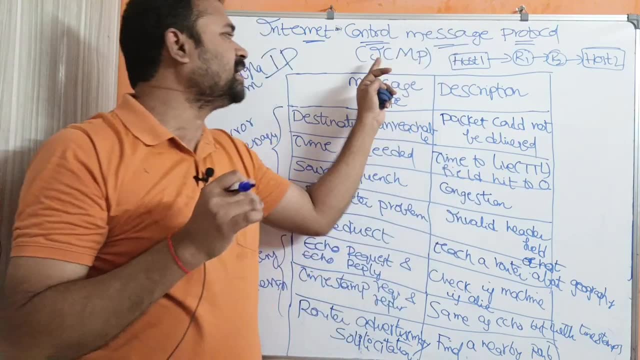 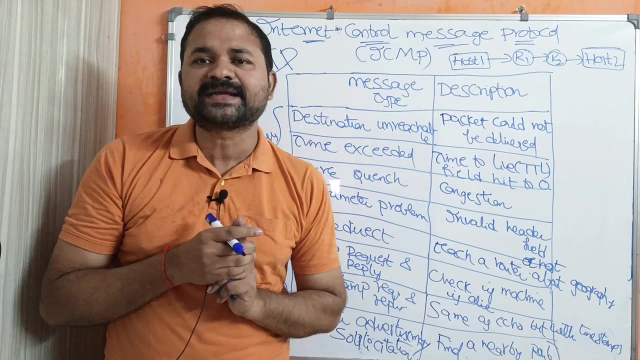 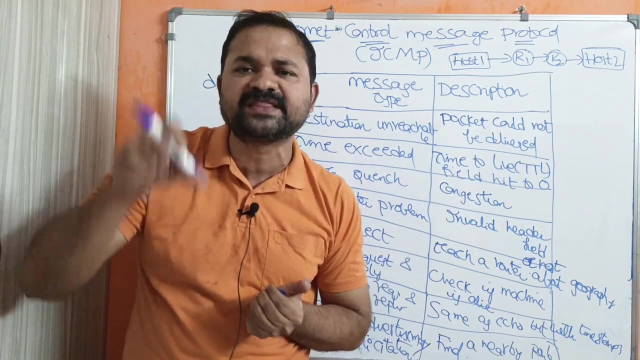 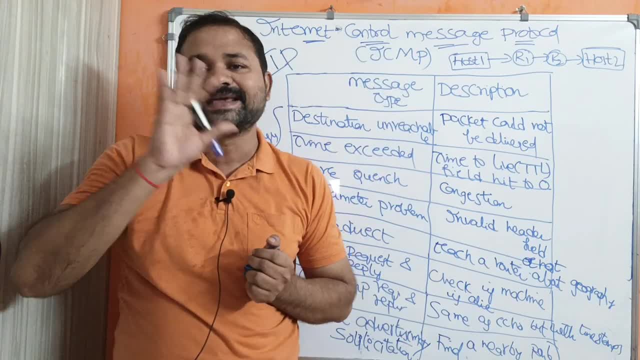 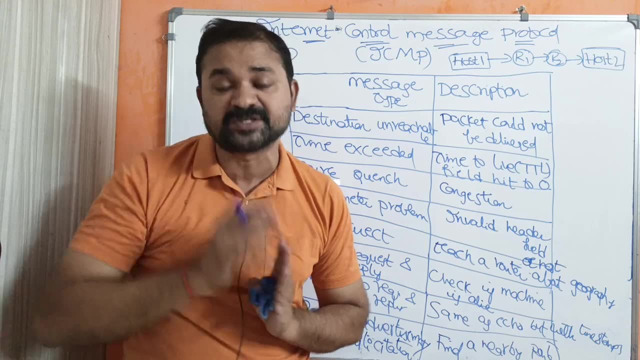 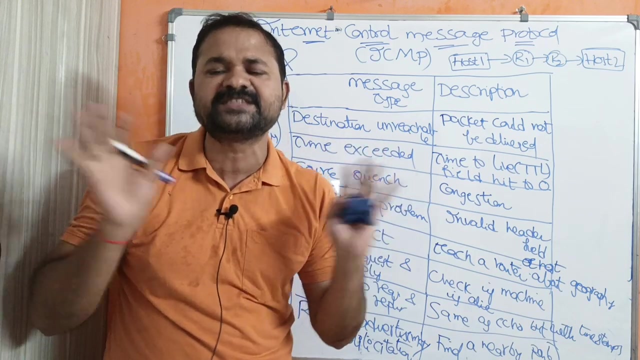 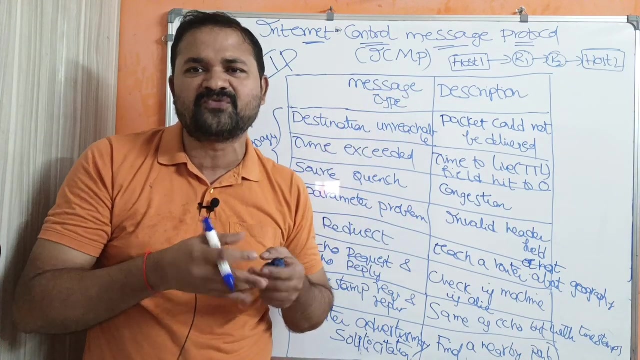 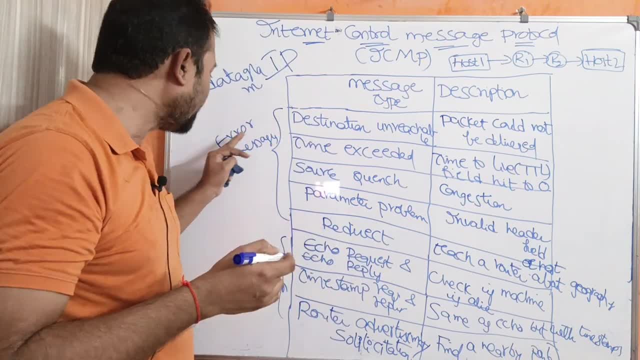 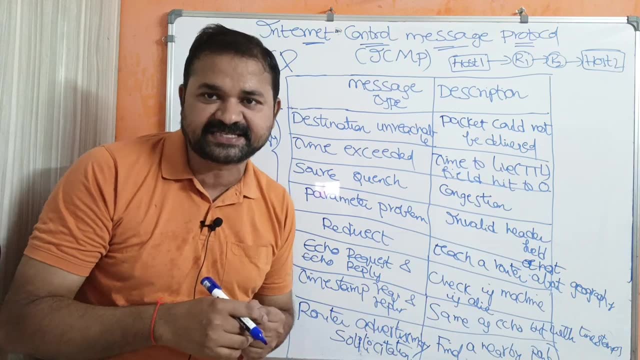 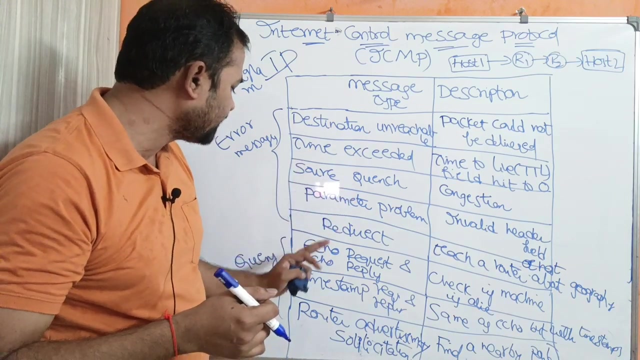 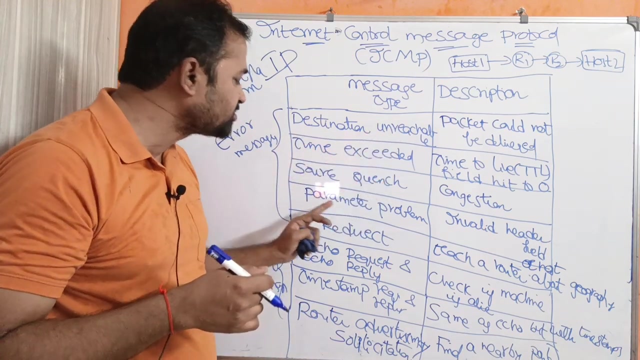 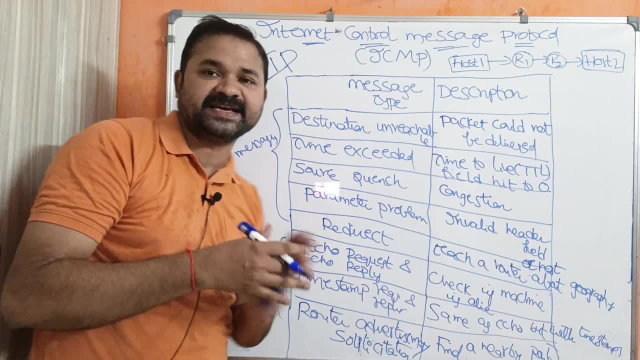 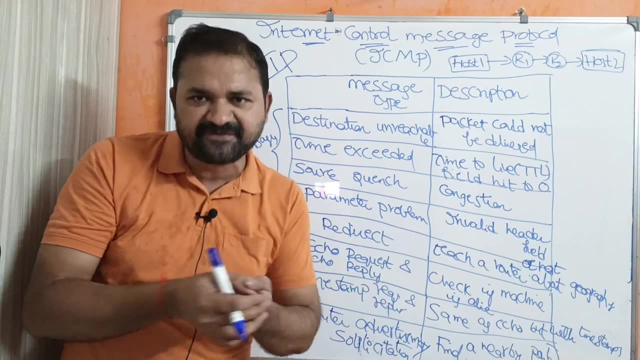 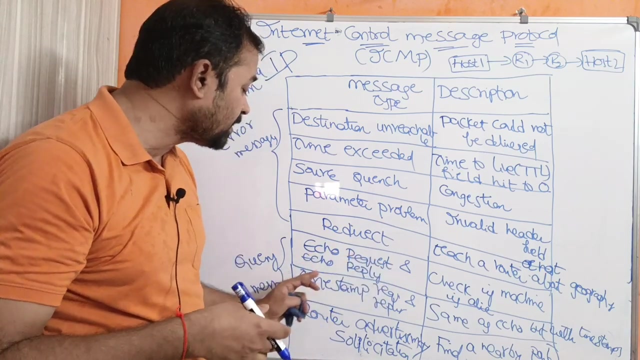 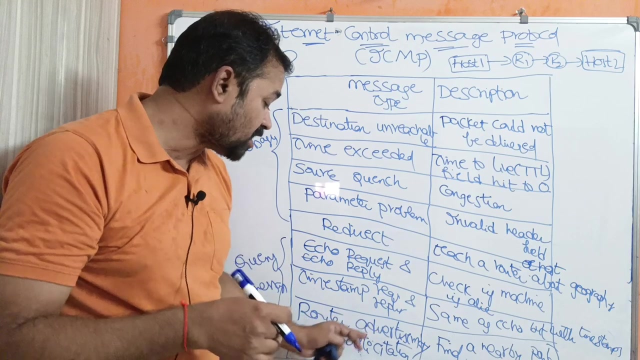 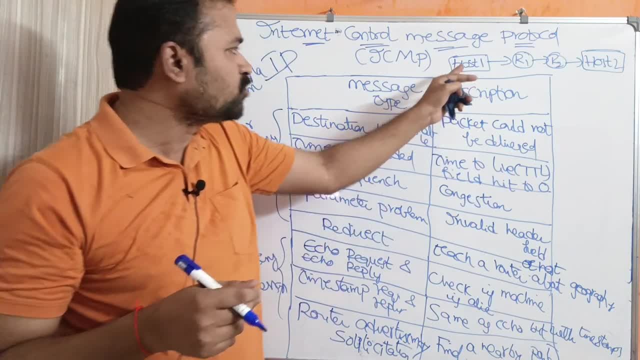 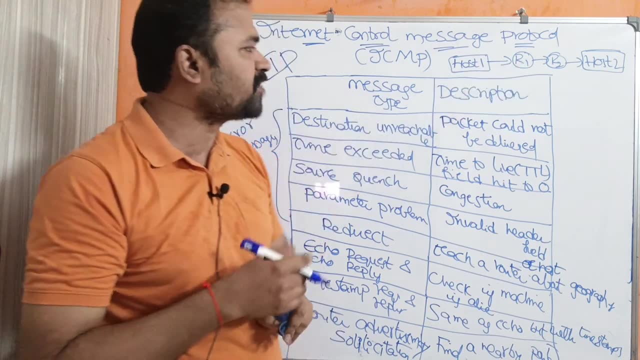 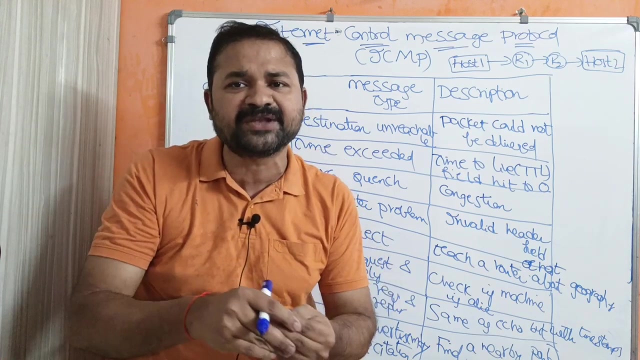 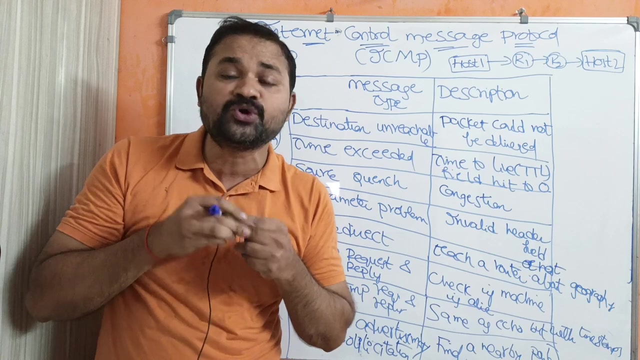 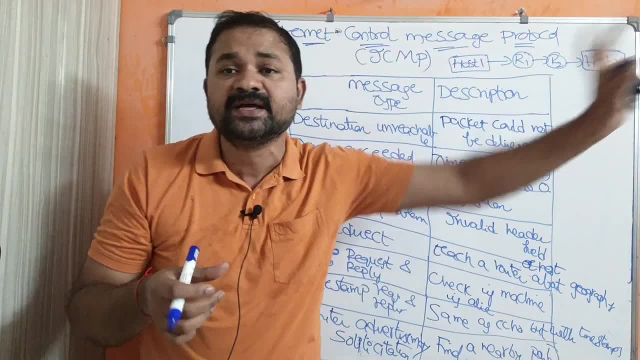 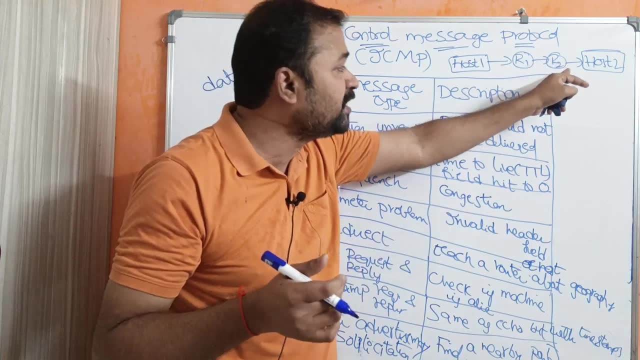 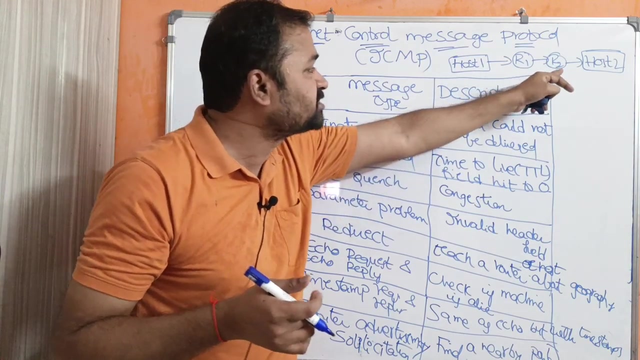 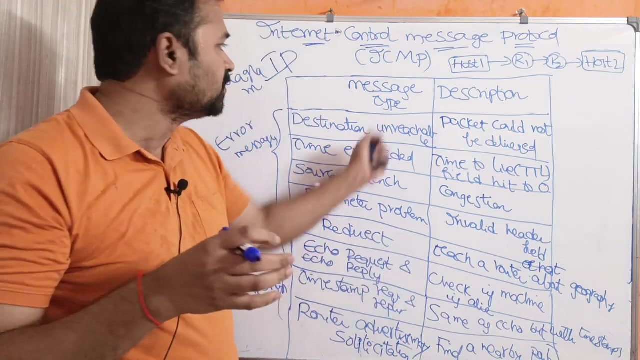 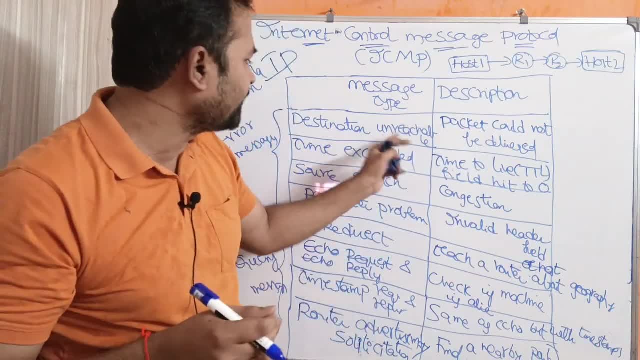 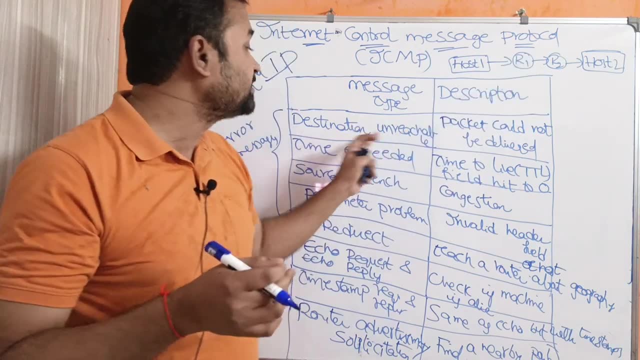 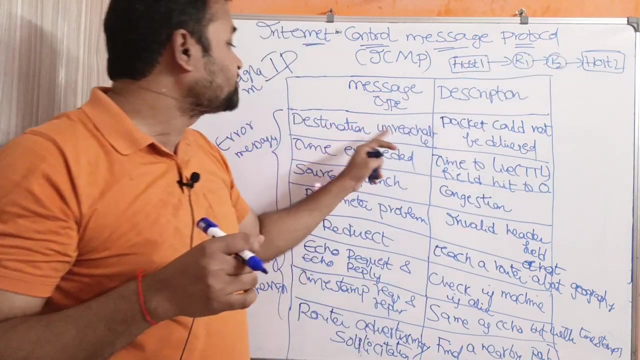 proper destination address. So here, what is the description about this? one Packet could not be delivered, So that is about destination unreachable. So here, R2 will discard that packet and R2 will send destination unreachable ICMP message to the host 1.. So host 1 after: 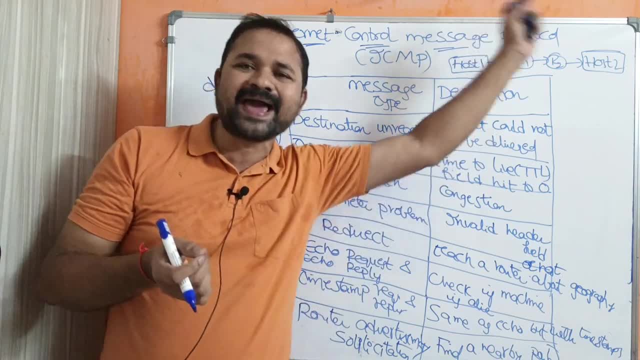 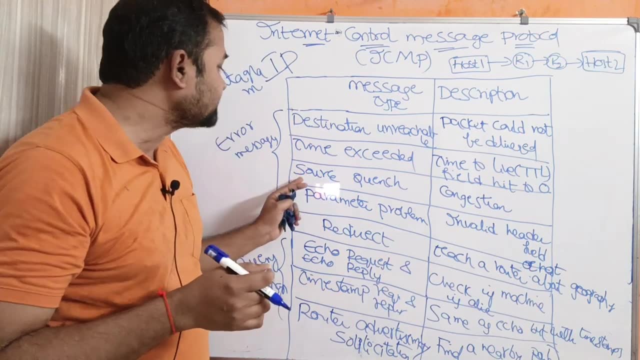 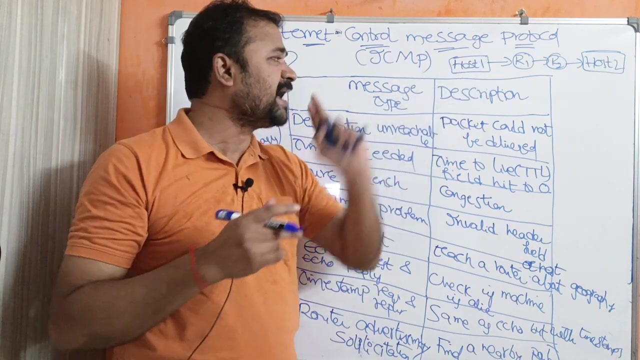 receiving that message, it will send one more packet with proper destination address to the corresponding destination host, And the second one is time exceeded. So what is the second ICMP message? Time exceeded. So here what will happen is every packet will have a time to leave field. 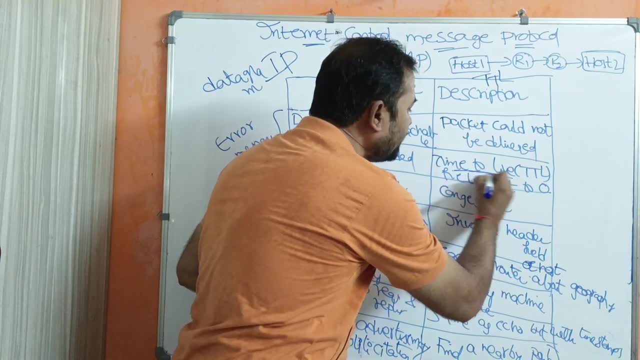 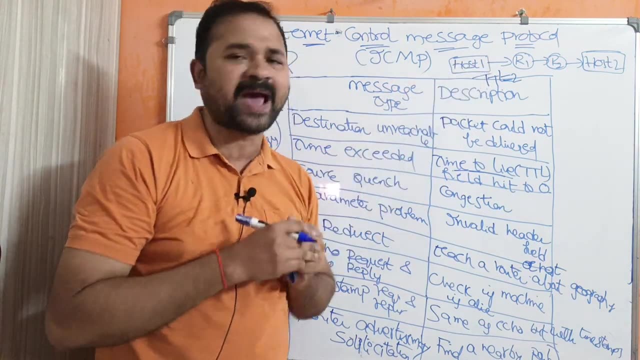 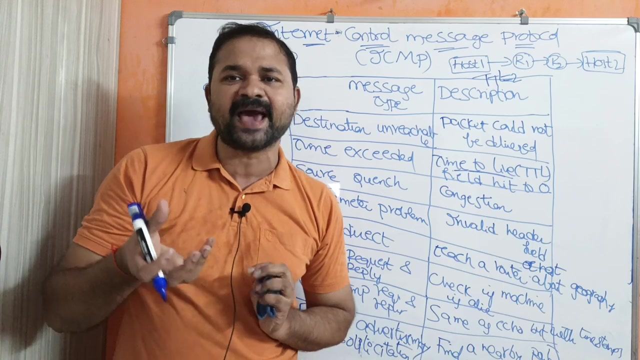 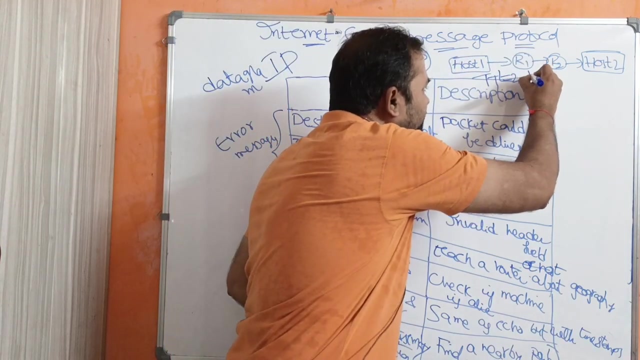 TTL. TTL stands for time to leave field, So let TTL field value is 2.. So here host 1 is transmitting a packet with TTL value 2.. So now R1 receives the packet. Upon receiving the packet, R1 decrements TTL field by 1.. So now the packet, TTL field will: 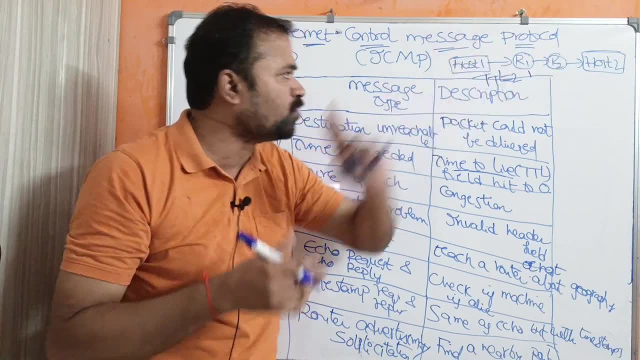 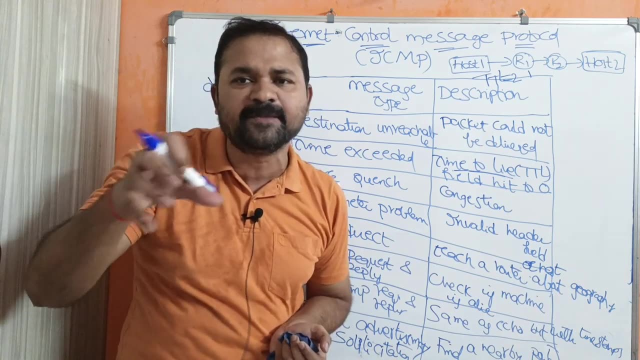 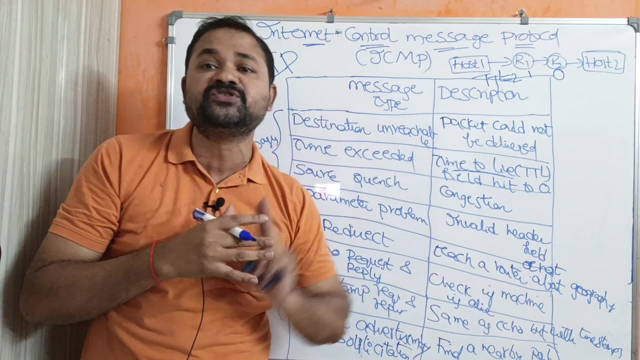 become 1.. So now R1 transmits the packet to R2.. Here, upon receiving the packet, the router or host will decrements time to leave field by 1.. So now the time to leave field will become zero. so whenever ttl value will become zero, then the corresponding 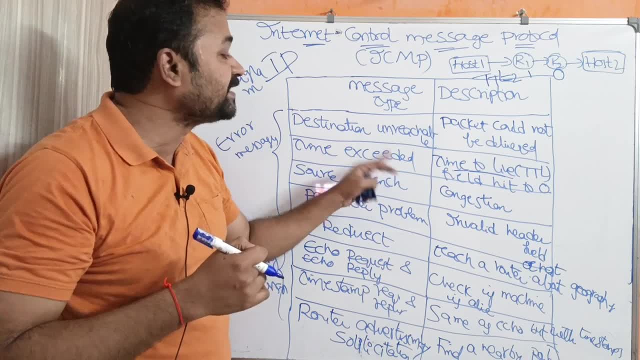 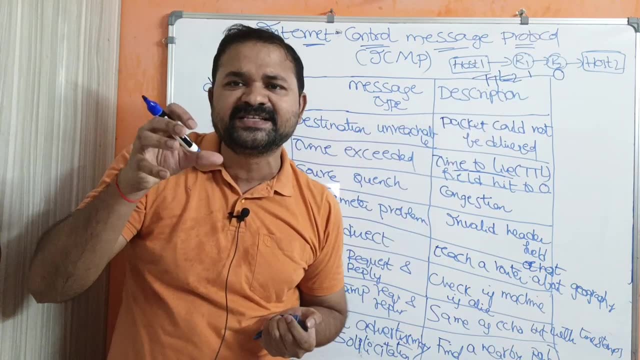 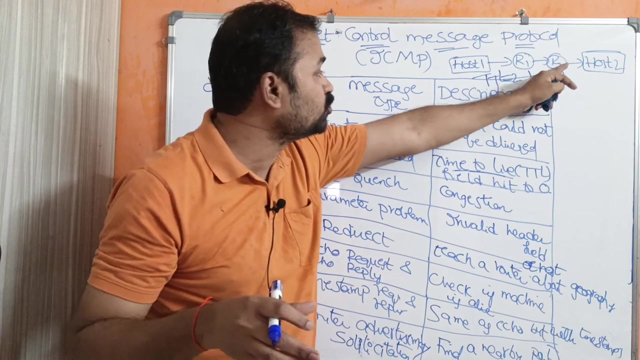 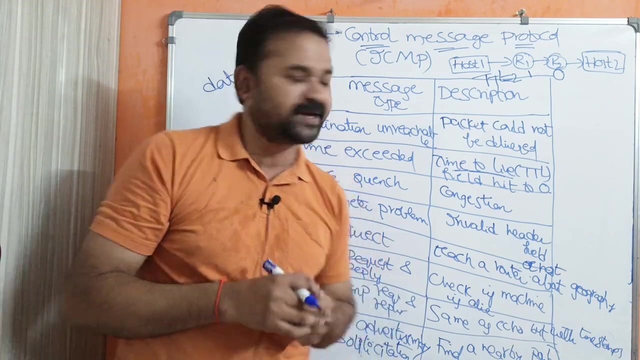 router will sense time exceeded icmp message to the host. so whenever time to leave field becomes zero, then the router will simply discards the packet and sends time exceeded icmp message to the host one. so now it is the responsibility of host one to transmit the packet one more time. okay, so. 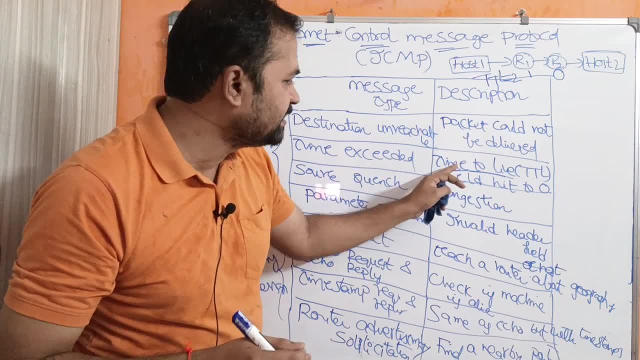 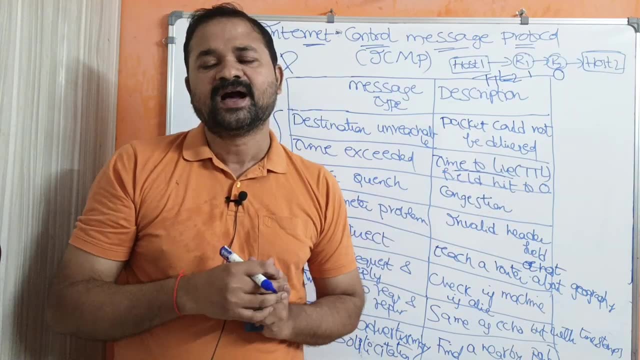 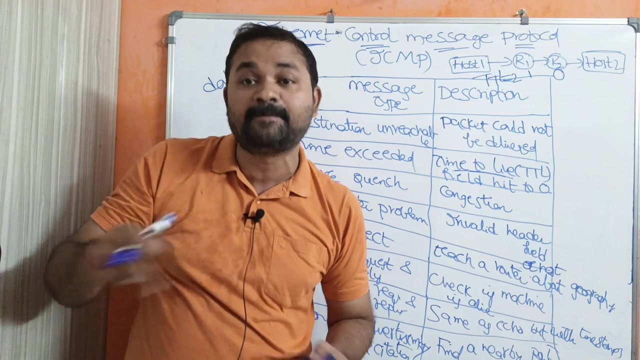 this is the first reason. so let's see the reason here. description here: time to leave ttl field hit to zero. and one more reason is: let me have a large packet. now that large packet will be trans will be fragmented into several parts. so let me have a large packet, so this packet is fragmented into. 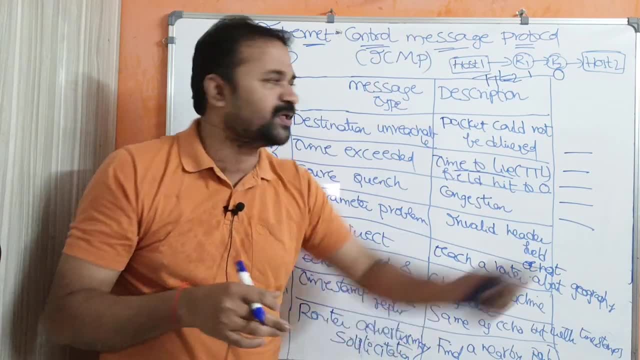 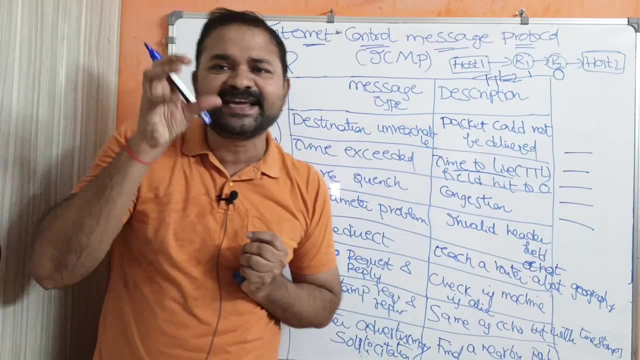 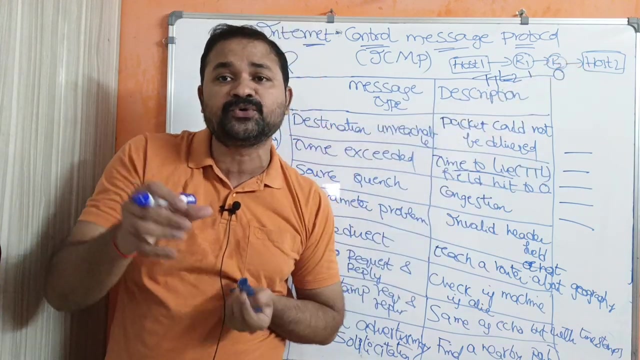 five smaller packets, but all those packets belonging to the same destination ip address. so whenever a router receives a packet then it will sets the timer. so all the fragments of the packet should reach to the router r2 within the time only. suppose if the timer expires that means 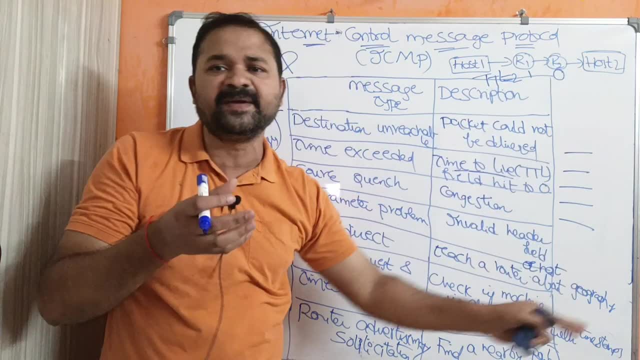 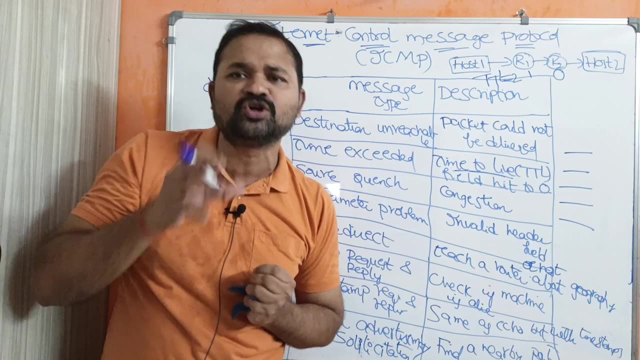 here. r2 is unable to receive all these fragments within the stipulated time period. so whenever the router is unable to receive all these fragments within the stipulated time period, so whenever the timer expires, then r2 simply discards all those fragments, all those fragments, fragments and sends time exceeded error icmp message to the host one. so host one has to transmit the packet one more time. so these are the two reasons why we why icmp time exceeded message will be generated. now let's see the third one: source quench, source quench. so this is generated because of two reasons. first one: 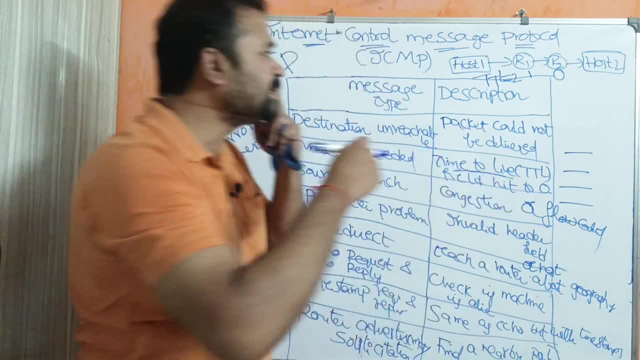 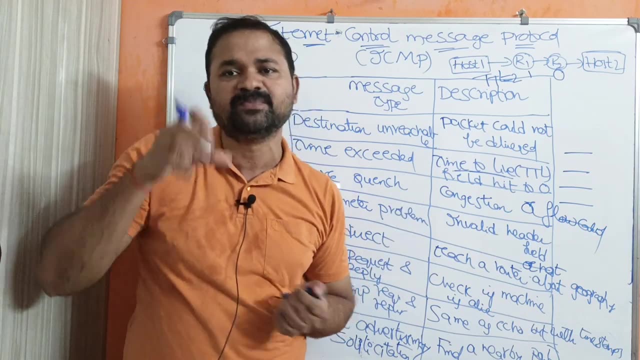 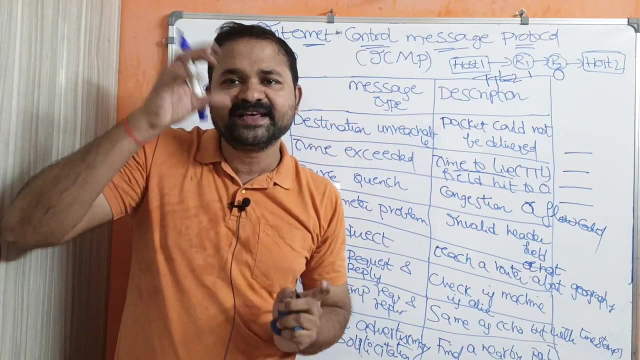 is congestion. second one is flow control. so let us assume that at router 2 there is a too much of traffic, there is a too much of congestion, so at this time router 2 sends source trench icmp message to the host one. so if there is a too much of traffic or congestion, immediately that router will. 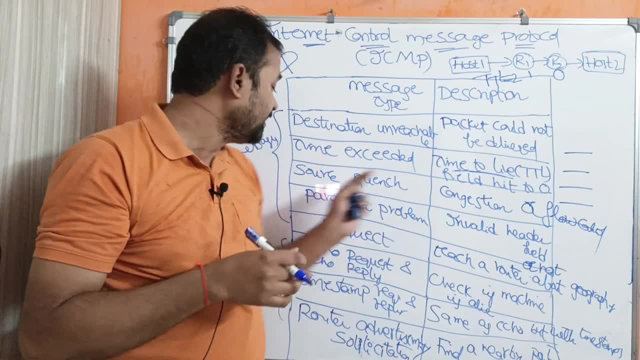 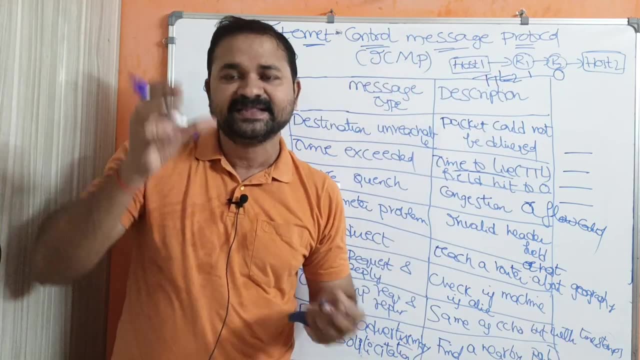 discard the packet. after discarding the packet, it will sense source quench error message to the host one. so by observing that, router 2 send source quench error message to the host 1. so by observing that message, host 1 knows that there is a too much of traffic at the corresponding routers. so 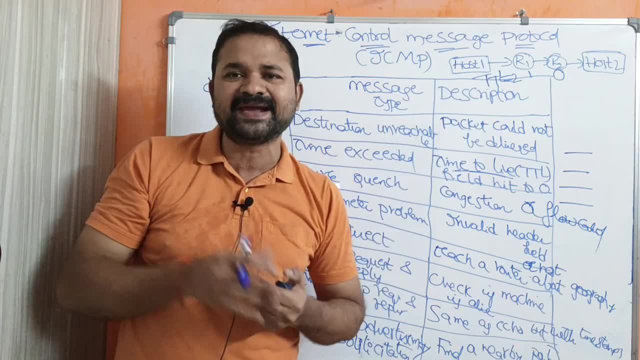 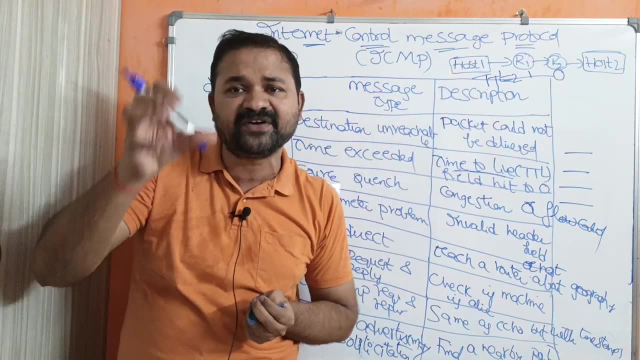 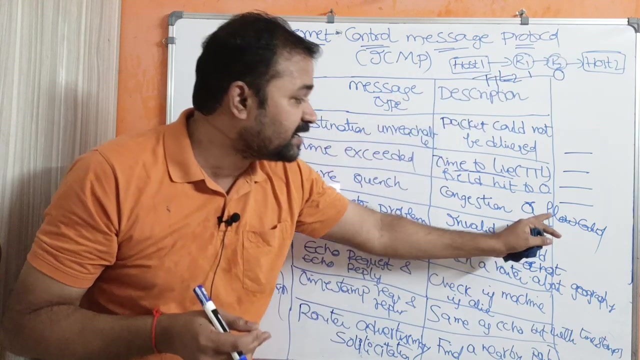 the corresponding host 1 will send one more packet, or it will wait for some time, because here there is a too much of traffic, so that's why the host 1 will wait for some period of time. so after that period of time it will send one more packet to the router 2, or there may be a possibility that 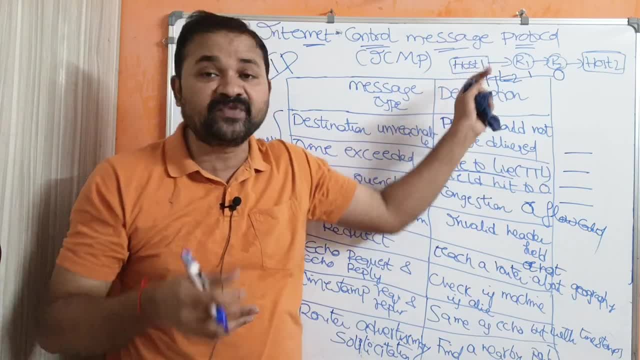 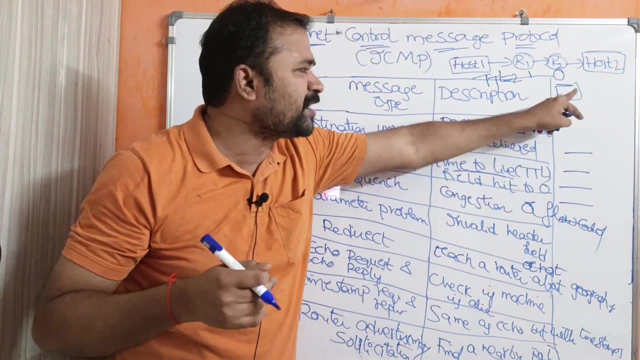 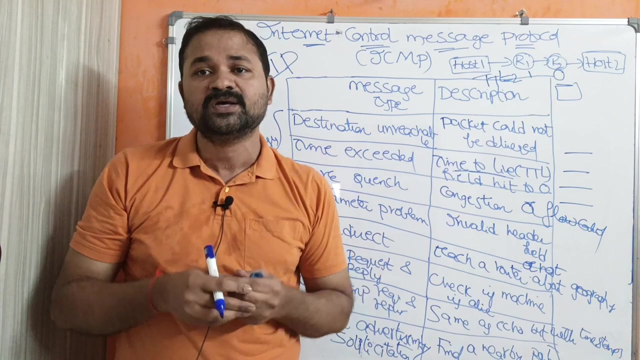 flow control. so flow control means here the host 1 is sending the packets at a faster rate, whereas at every router we will have some queue. but this queue capacity is very, very limited. so here router is unable to store all those packets in the queue. so because of that some packets may be lost. so 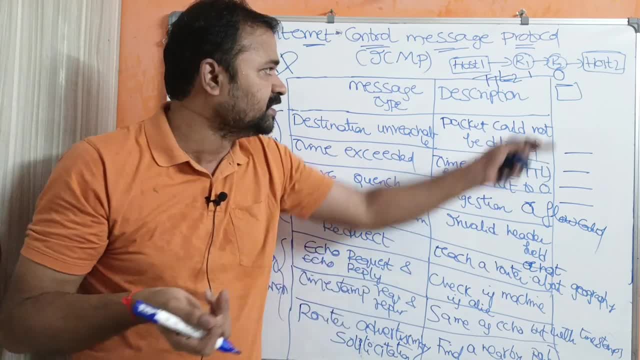 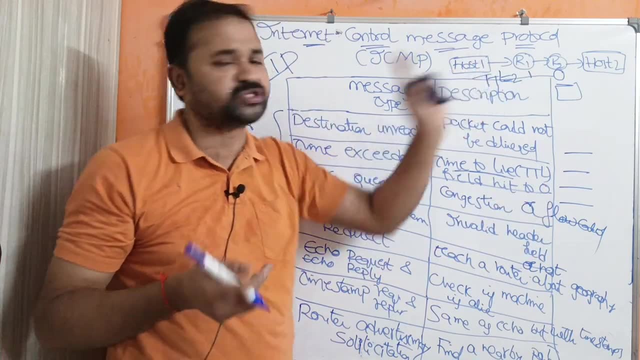 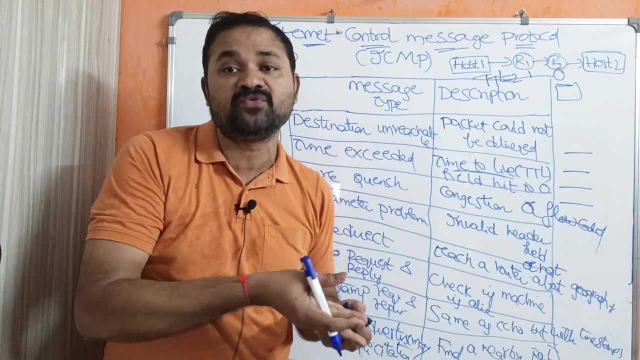 so whenever the packets are lasting discarding, then what will happen? router 2 will sense that congestion, that flow control icmp message to the host 1. so now host 1 will stops sending the packet for some period of time, will slows down for some period of time. after that it will sense one more packet to the router 2. 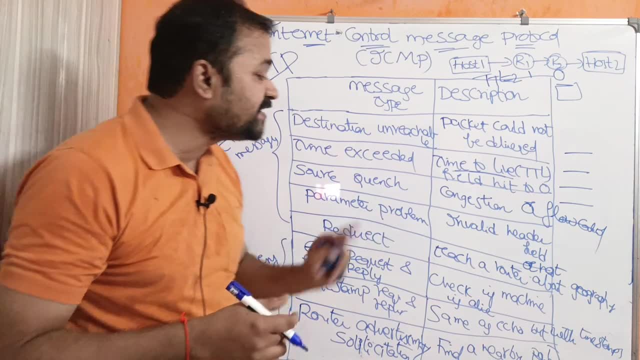 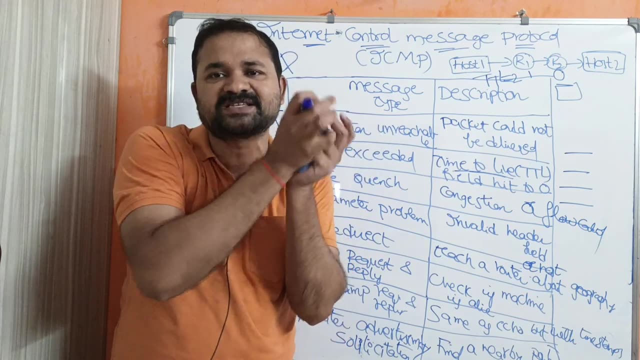 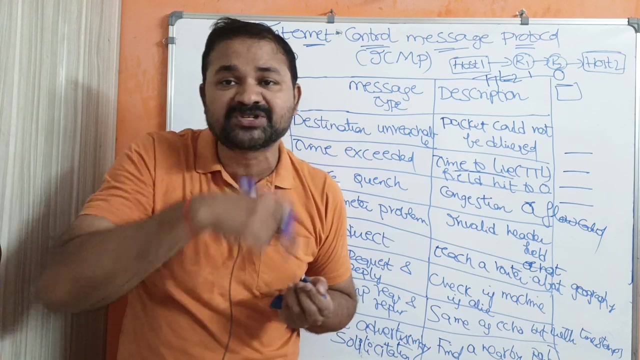 so this is about source quench and the next one is parameter problem. here the problem is invalid header field. so we know that every packet will starts with some header, every packet will have some header. so like there is a ambiguity in header field, so that means means some bits of the header field are modified. So at that time what will happen? Router will. 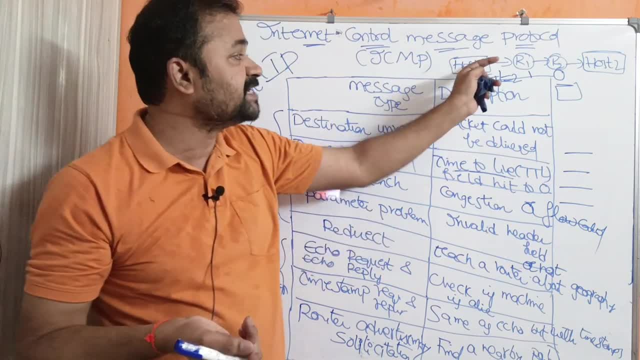 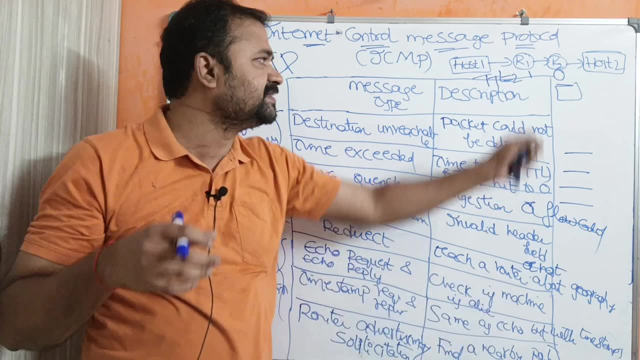 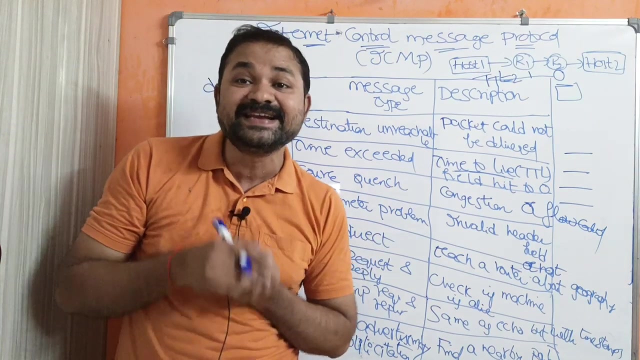 simply sends parameter problem ICMP message to the host 1.. So if there is a problem in the header field, so first router discards the packet. After discarding the packet it will send parameter problem ICMP message to the host 1.. And the next error message is redirection. Here host 1 wants. 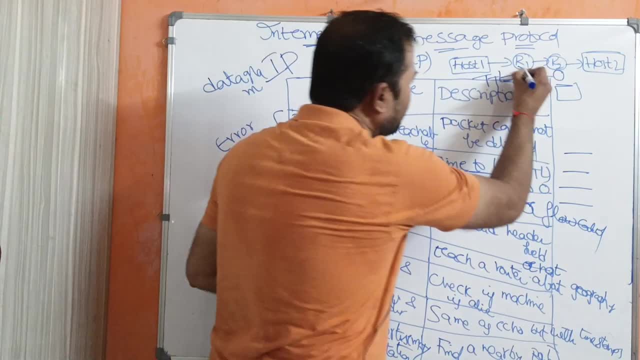 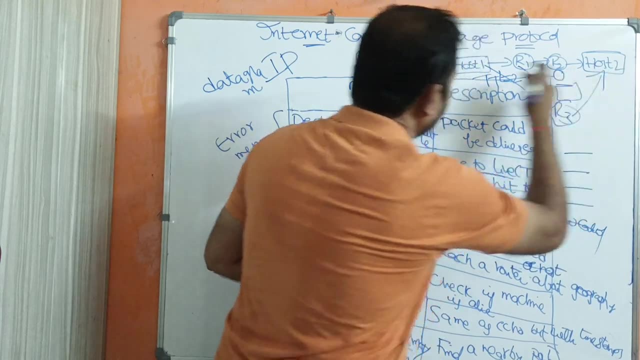 to transmit a packet to host 2.. But let we have here different paths. here Host 1 can send like this also. So here what is the first part? Host 1 is sending the packet to R1.. R1 sends the packet. 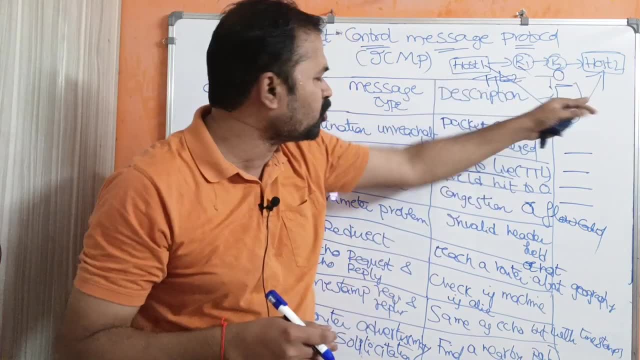 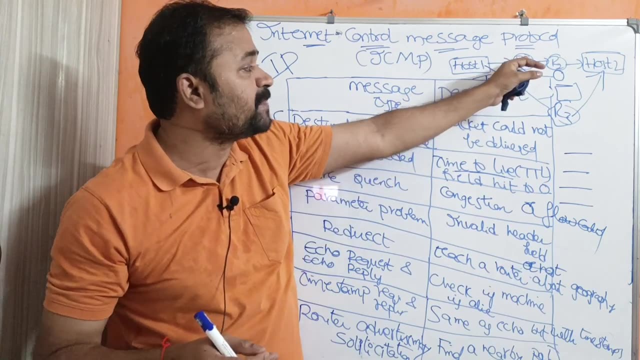 to R2.. R2 sends the packet to host 2.. We have one more path. Host 1 can send the packet to R3.. R3 can send the packet to host 2.. Let host 1 transmitted the packet to R1. But R1 knows the. 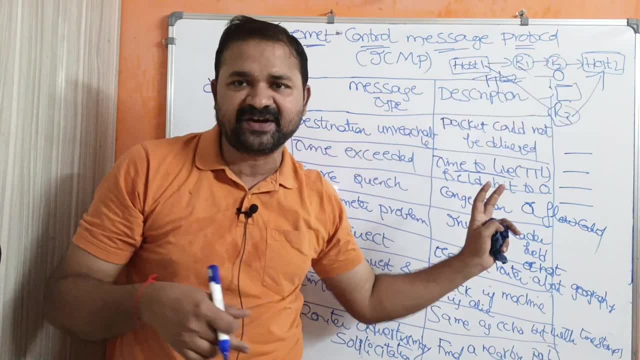 complete geography of the packet. So R1 can send the packet to R2.. R2 can send the packet to R3.. R2 can also send the corresponding network. Why? Because every router will have routing table. Routing table provides the information about the nearest. 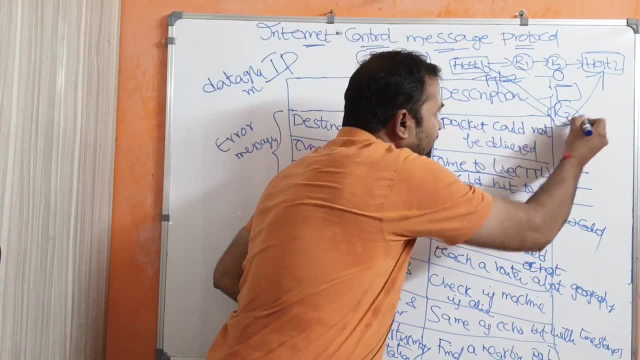 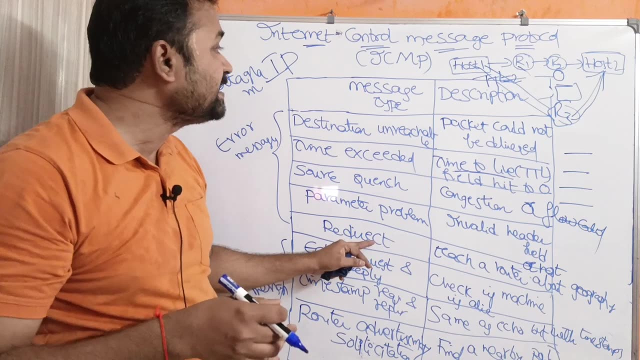 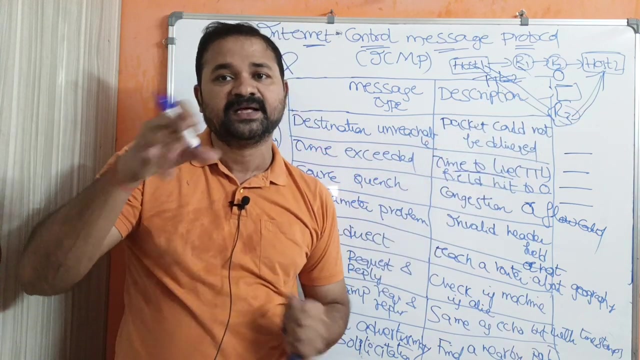 routers also. Let us assume this is the best path in order to transmit the packet. So once R1 receives the packet, it discards that packet and sends redirect ICMP message to host 1.. So that message will contain that R3 is the best path in order to transmit that packet to the host 2.. So, after remarking R2, turns R3 to R1.. After remarking R2, takes the packet from R3 to host 2.. After remarking R2, takes the packet from R3 to R2.. So, after remarking R2, takes the packet from R2.. So, after 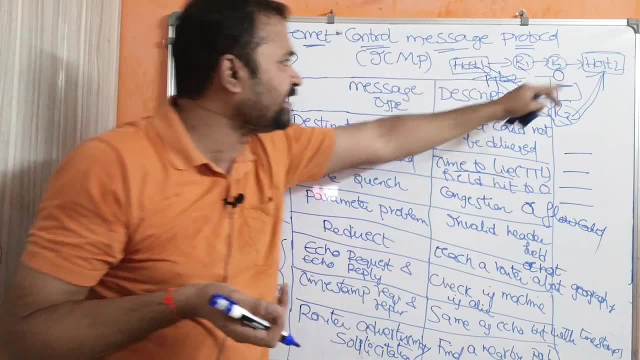 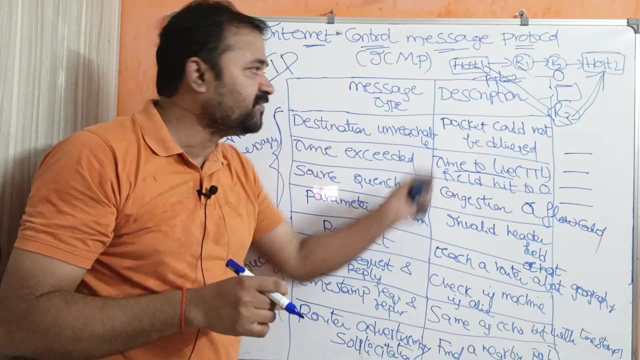 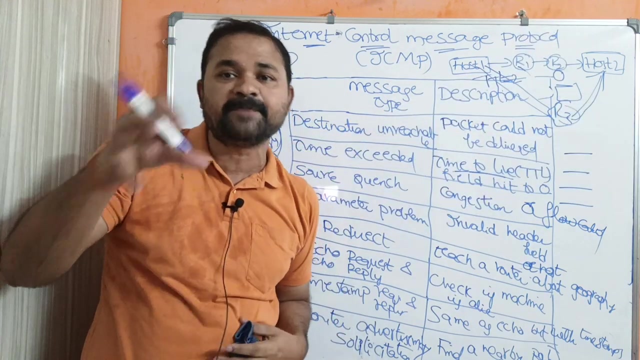 after observing, after reading that message, host 1 can transmit the packet to host 2 via r3. these are the error messages. okay, so whenever an error occurred, then the immediate, then the intermediate routers or intermediate host discards the packets and after discarding the packet, it. 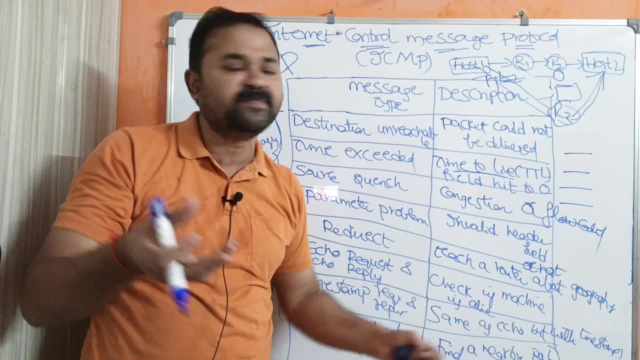 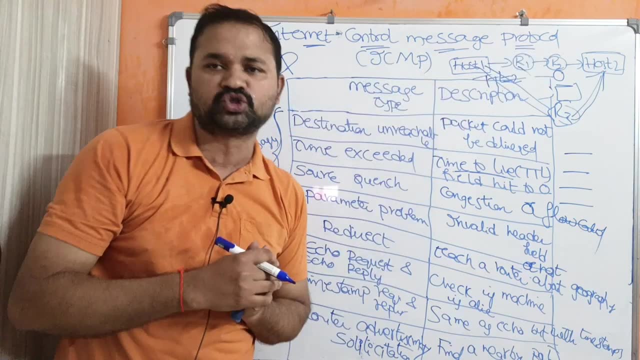 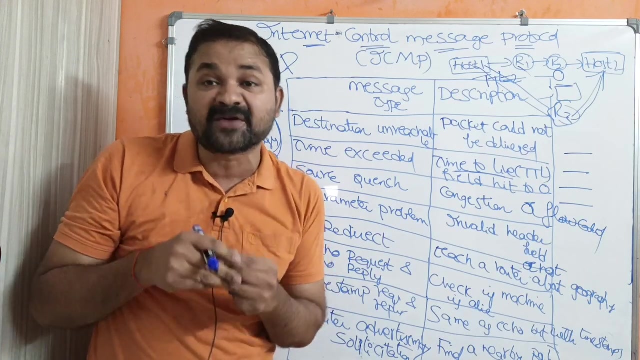 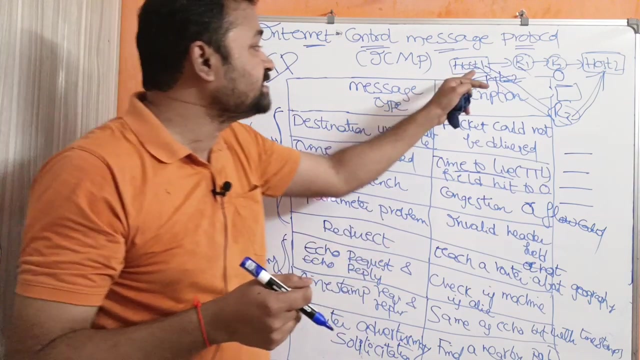 provides a corresponding error error icmp message to the source host. so now source host can provide another packet to the corresponding host to 2, whereas the remaining three are query messages. so these are mainly useful in order to know about the performance of the network. okay, so the first one is echo request and echo reply. so let us assume that host 1 wants to. 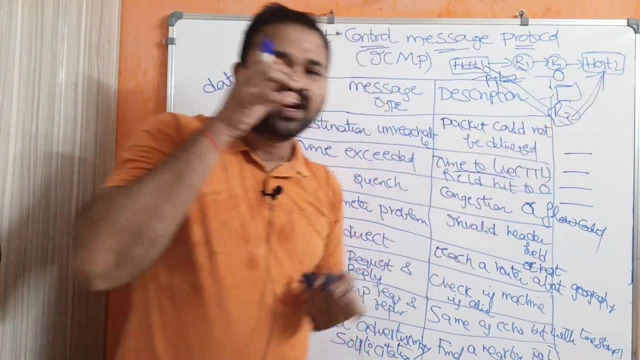 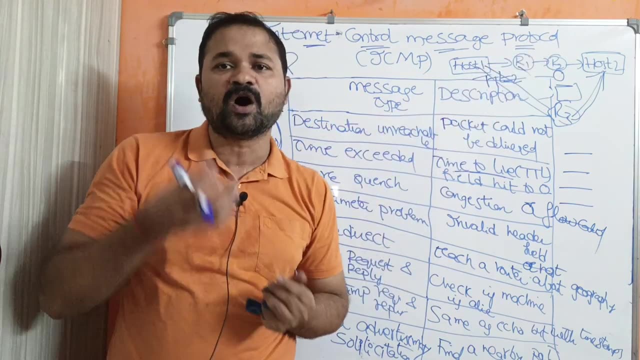 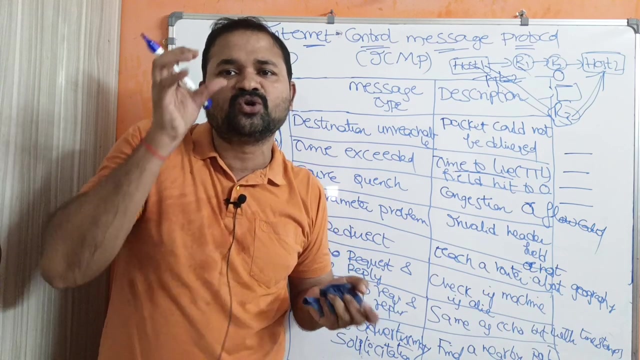 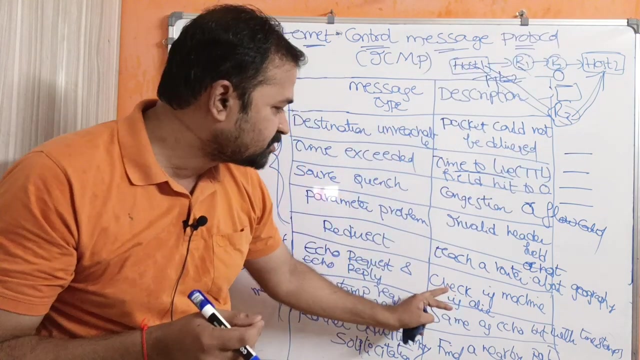 wants to know about whether host 2 is alive or not. so for that purpose host 1 can send echo request to the host 2. so upon receiving the echo request message host 2 can sense echo reply message to the host 1. so once host 1 reads that echo reply message, then host 1 comes to know that host 2 is alive. so check if the 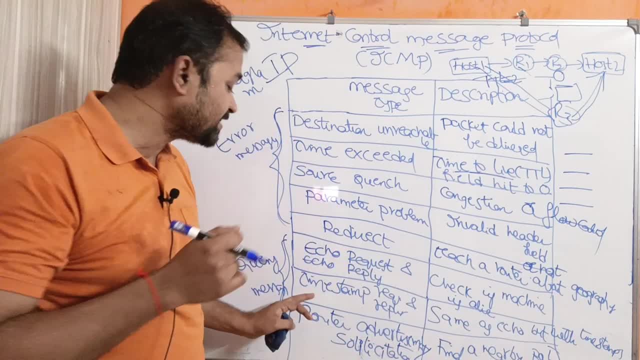 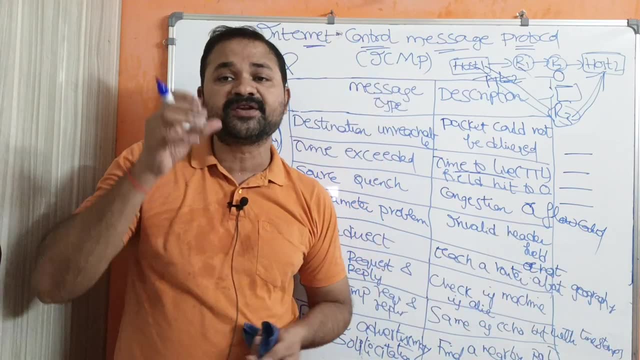 destination: check if the mission is alive or not. and the next one is time stamp: request and reply: same as the echo, but with time stamps. so, in order to know the performance about the network, okay, let a host 1 be able to know the performance of the network. okay, let a host 1 be able to know the. 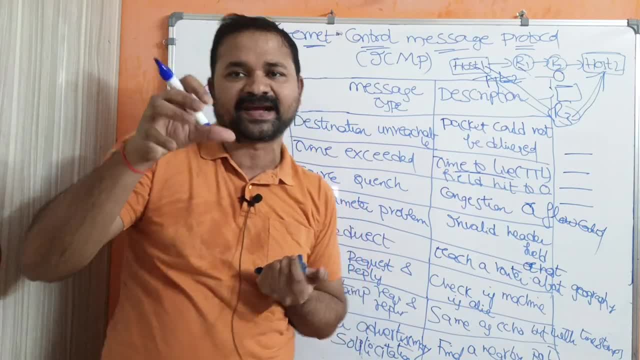 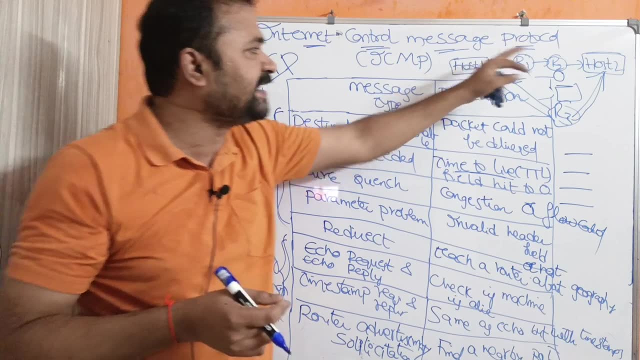 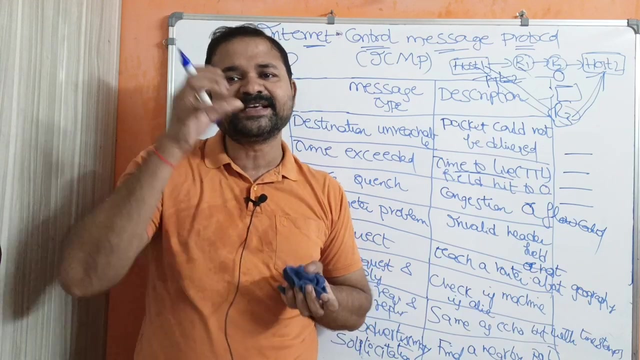 how much time it will take for transmitting a packet to host 2. so in order to know about how much time it will take, so it will sense a time stamp request to host 2. so upon receiving that, host 2 will provide time stamp reply to host 1. so it is mainly useful for how much time.